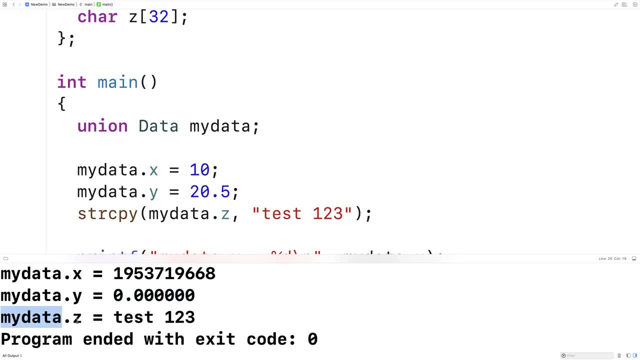 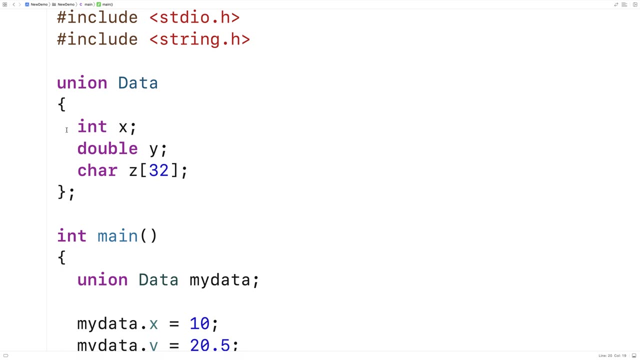 mydatay looks like zero and only mydataz actually has what we expected stored into it. So what's going on here is the key difference between how a union works and how a struct works. With the union, we only have enough space to store one of these things at a time. 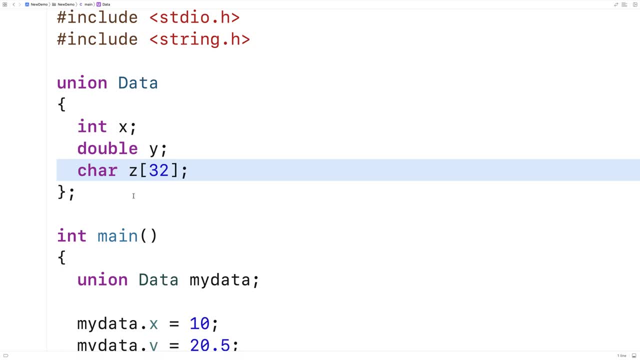 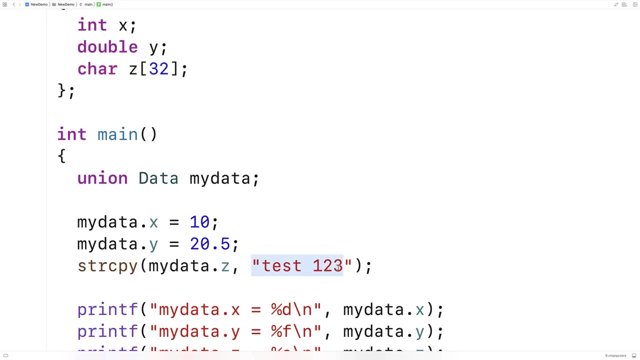 and they actually all occupy the same space in memory. so when i actually copied in this string test123 into mydataz, this actually overwrote the 20.5 that was previously stored in that same spot in memory as a double value and we set mydatay equal to 20.5. 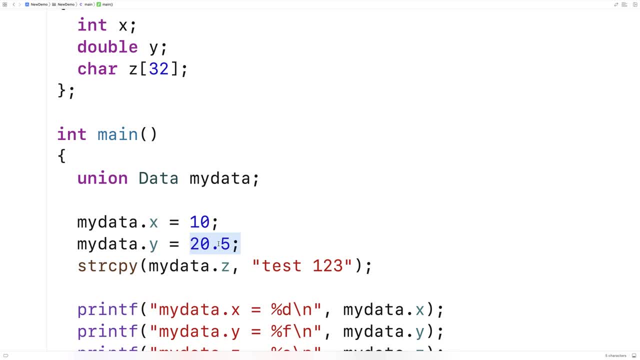 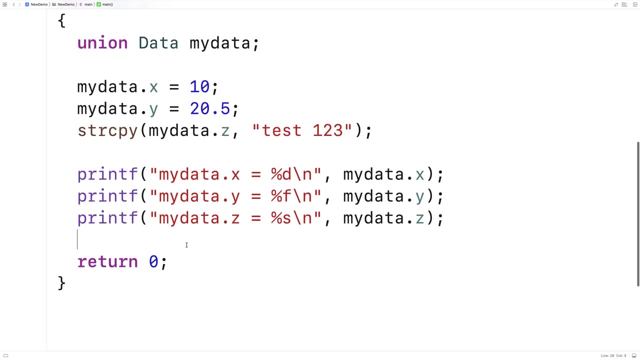 that overwrote what was previously stored in memory at the same location when we set the number x to 10, because they all occupy the same space in memory. so if i were to set one of these individually and then print it out, it would work fine. so here, if i said mydatax is equal to 10, 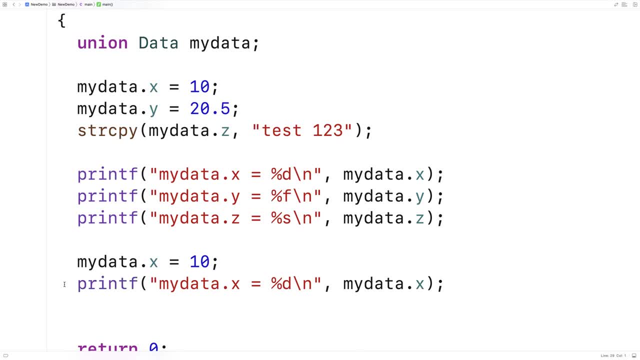 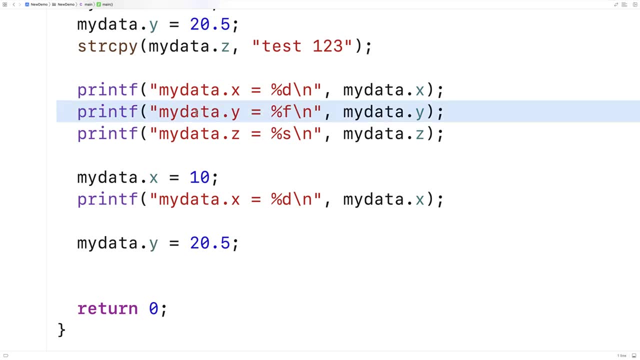 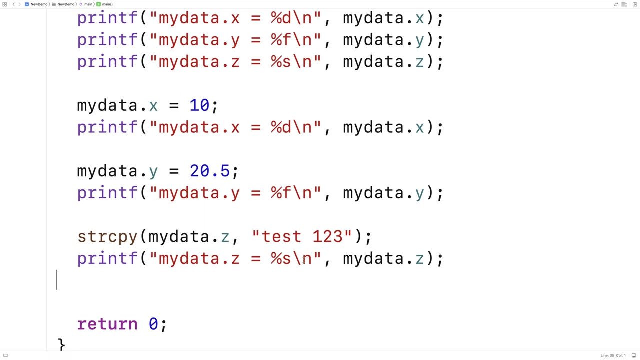 and then i did a printf of mydatax. it'll be okay. then after that i'll set mydatay equal to 20.5 and then i'll printf mydatay and then, finally, i'll string copy test123 into mydataz and then i'll printf mydataz and this should all work okay now? so if i run this, 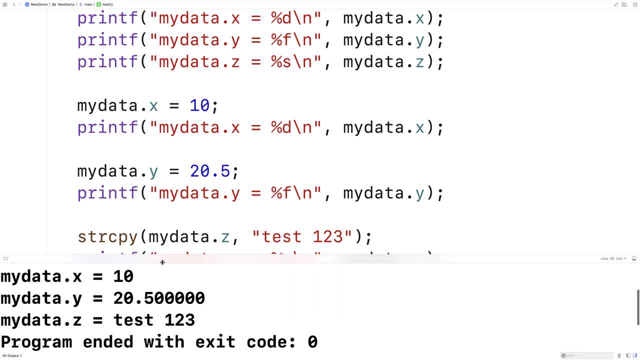 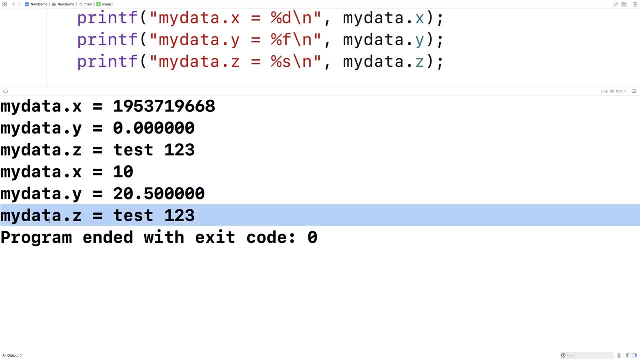 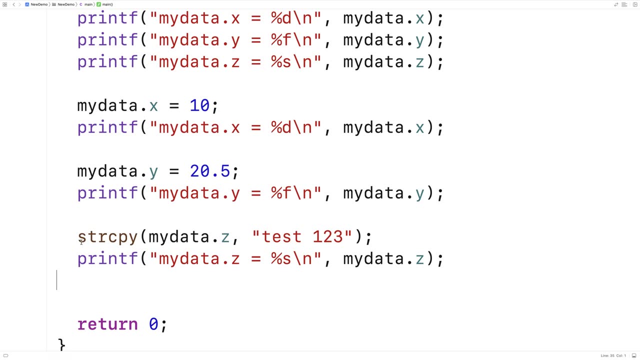 version here, you'll see that we actually do get them printed out. okay, so now we get: mydatax is 10, mydatay is 20.5 and mydataz is test123. so with a union, we can only use one of the members at a time, because all of the members occupy the same space in memory. 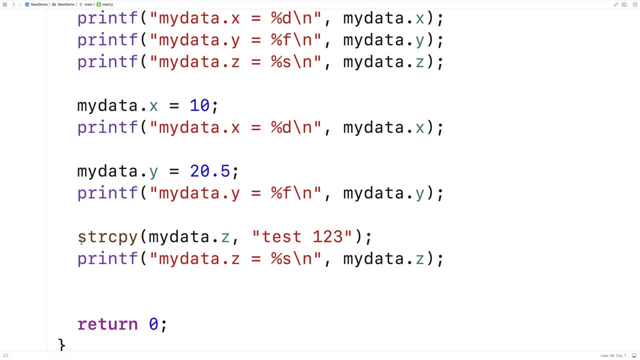 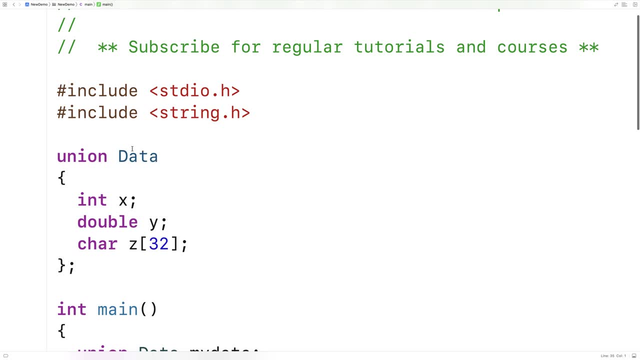 and if we set one of them, we're going to be effectively overwriting the other one. now because they all occupy the same space in memory. the space that it takes to store a union is going to be the size of the largest member in the union and in this case, here, that's going to be the 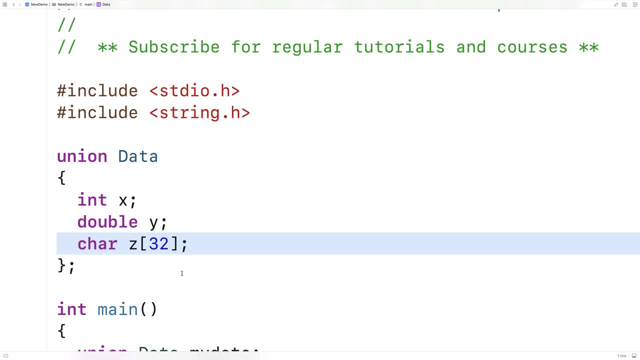 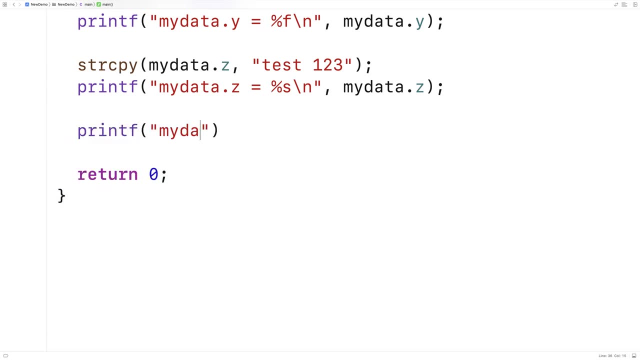 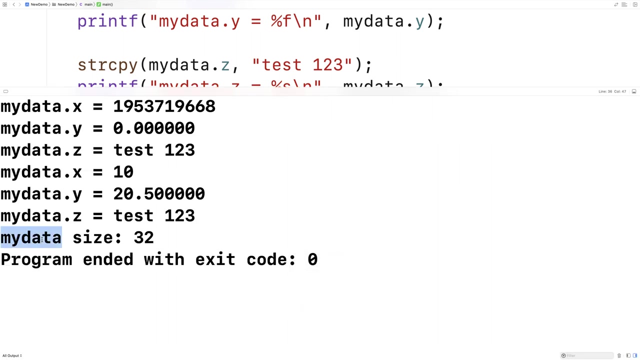 character array z that stores the largest member in the union and in this case here that's going to store those 32 characters. so here we'll print it out. we'll say printf- mydatasize%d, slash n and we'll output the size of mydata. if we save this here and run it, we get that mydata has a size of. 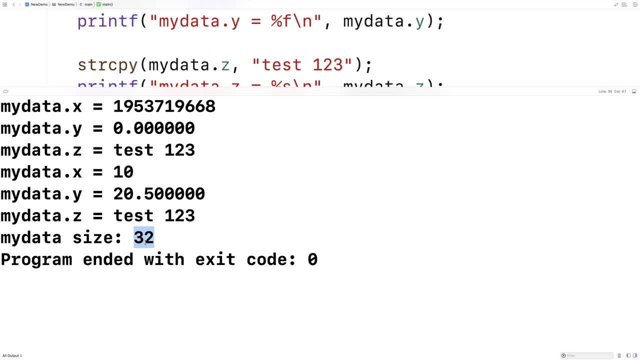 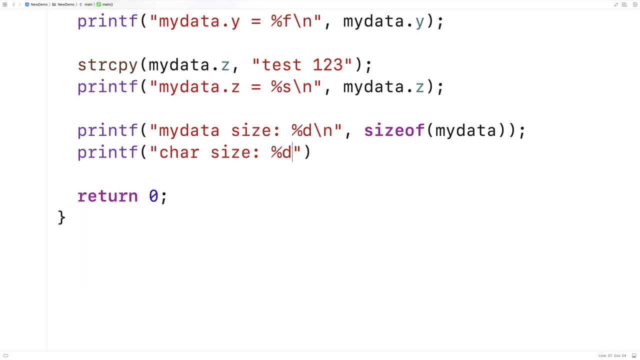 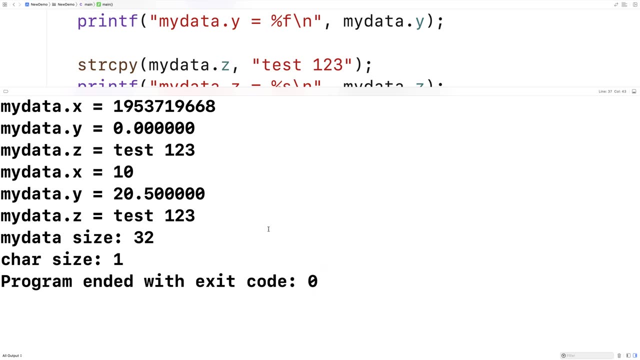 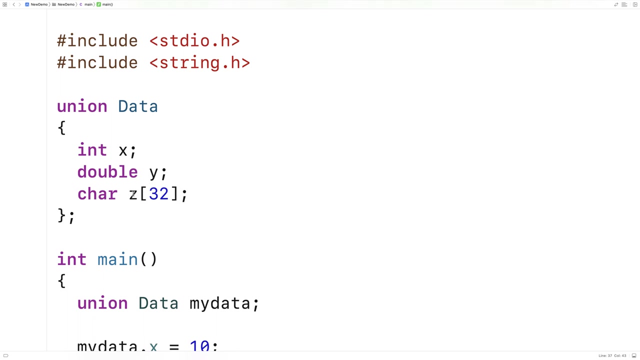 32, and that's because we need 32 bytes to store those 32 characters of the z character array. so if i say here printf- car size, percent d slash n, and i do size of car, we're going to find that it takes one byte to store a character. so that's why mydata as a whole takes up 32 bytes, because 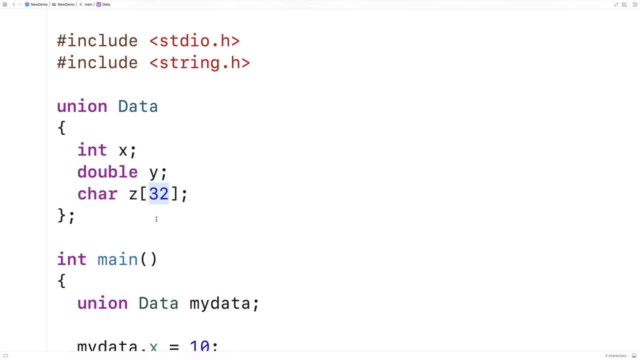 this character array z is 32 characters long. one byte per character leaves us with 32 bytes required to store any one of these members. now, a double and an int will take up less than 32 bytes, but that doesn't matter because you potentially have to store. 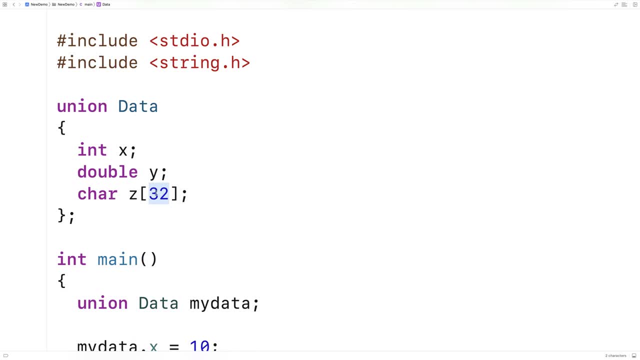 a 32 character array as part of this union. it doesn't matter, these take up less space, the whole thing still has to occupy 32 bytes of memory. so why we would use unions is basically because we could save space. so if we only have to store one thing at a time- but we know it's- 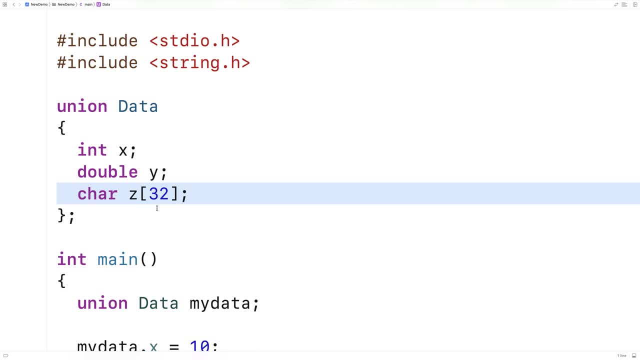 going to be one of several things. we could create a union of those things, knowing that only one of those is going to be in use at any given time, thus taking up less memory than if we had a struct, where a struct is going to go out and create space for all of those things. 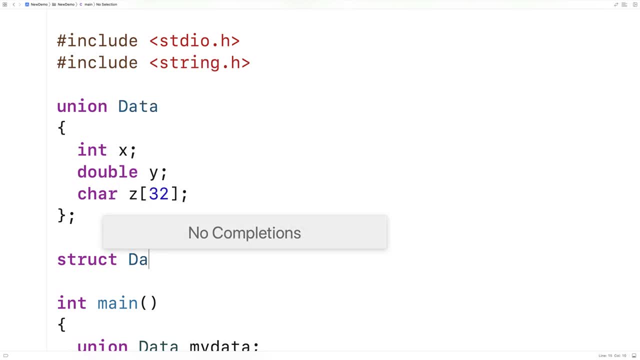 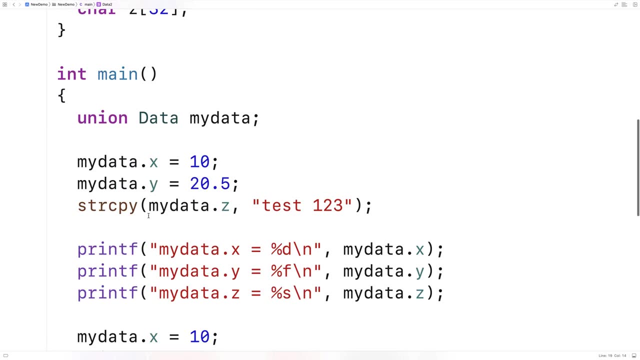 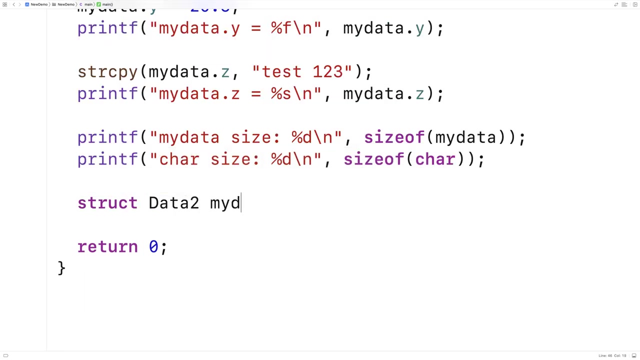 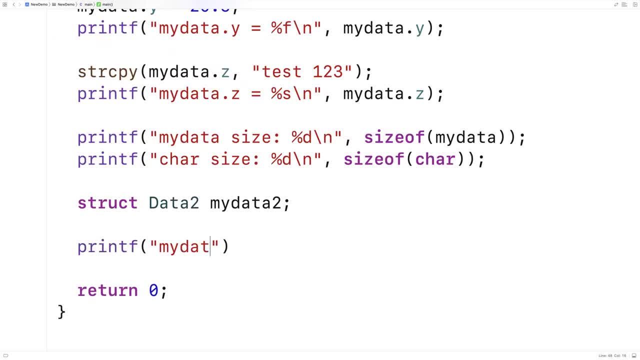 and then down here i say struct data 2, mydata 2, and then down here i say struct data 2, mydata 2, and we do a printf of mydata2 size, %d, slash n, and we output size of mydata2. we're going to find that it's more than 32. 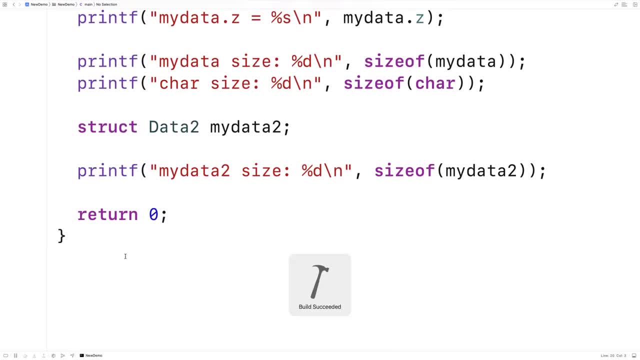 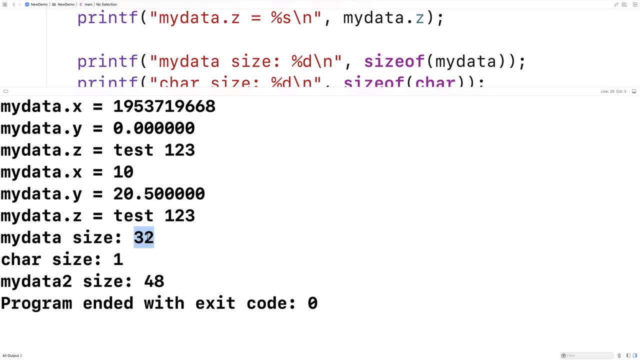 forgot a semicolon there, but we're going to find out that it's more than 32. it's going to be 48, because in addition to storing the 32 characters, we've also got to store an int and a double. so next up, let's talk about pointers to unions. 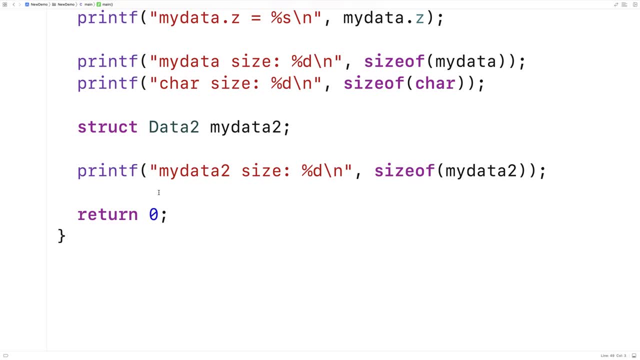 so pointers to unions work a lot like pointers to structs. so here, if i said union, data, star pointer is equal to and mydata. what i have here is a pointer to a union and i've set it equal to the memory address of mydata if i want to access the members of mydata. 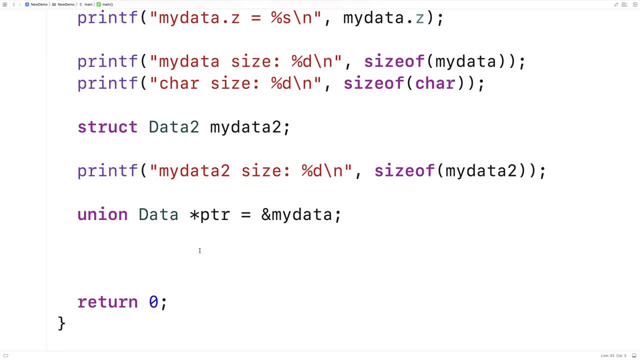 i can do so using mydata, using the arrow notation, just like i do with a struct. so i could say: printf: pointer z is equal to %s, slash n. and i can access the member variables of the union being pointed to by this pointer by saying pointer arrow z. 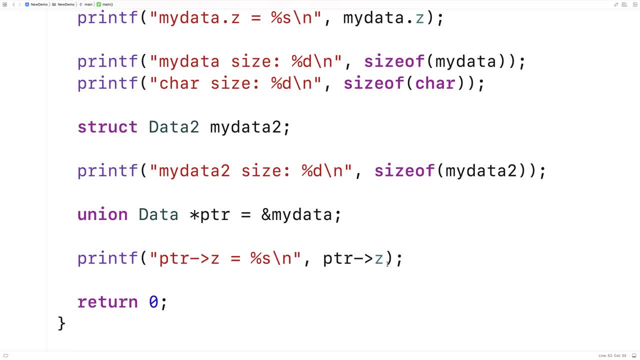 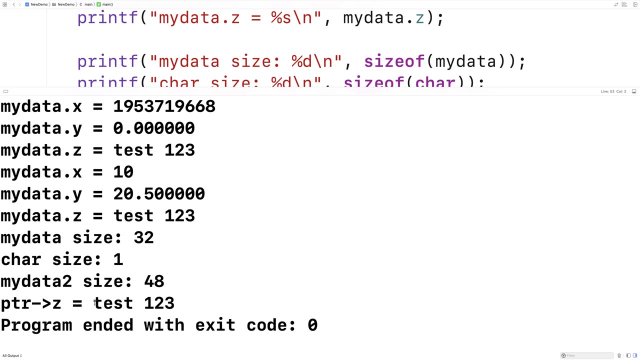 so this here is the arrow notation and it allows us to get at the members, in this case z, of the union that the pointer is pointing to, in this case mydata. so if i run this, we should get a printout of test123, because that's what the pointer is pointing to. 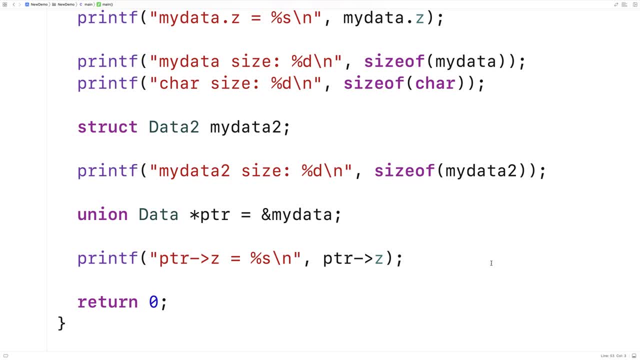 in terms of what the union is storing there. so, because unions typically only store useful data for one member at a time, we really need to know which member is active, like which one is really being used, and so a common pattern is to see a struct wrap a union. 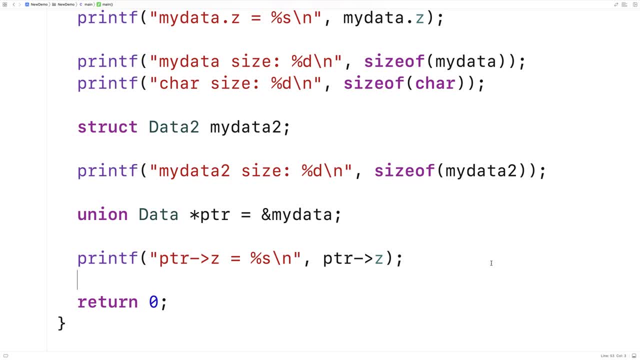 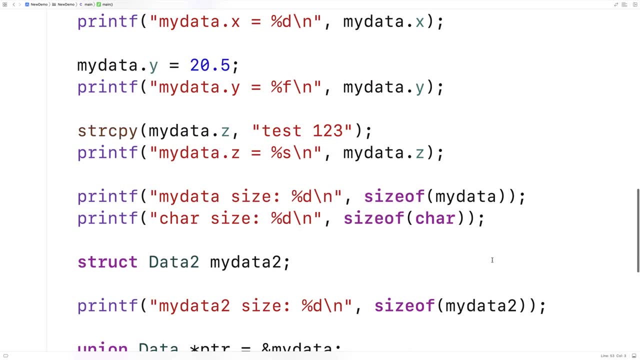 in the sense that it's not a union, but it's a union in the sense of having it as a member and the struct can include a member. that signifies which of the union members is actually being used. so for example, up here we could say typedef- struct. 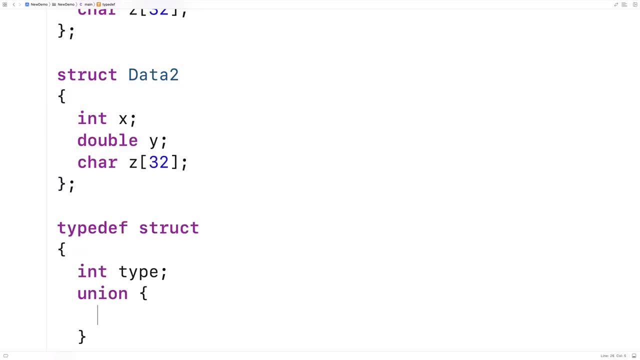 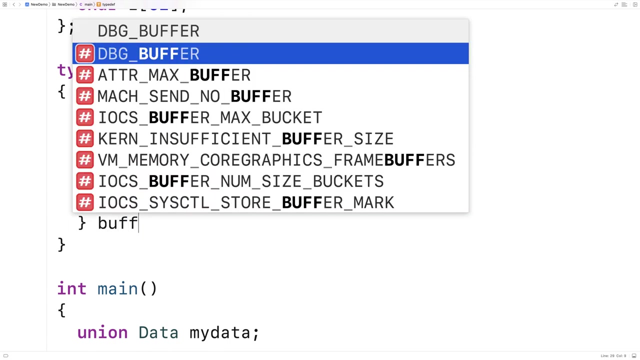 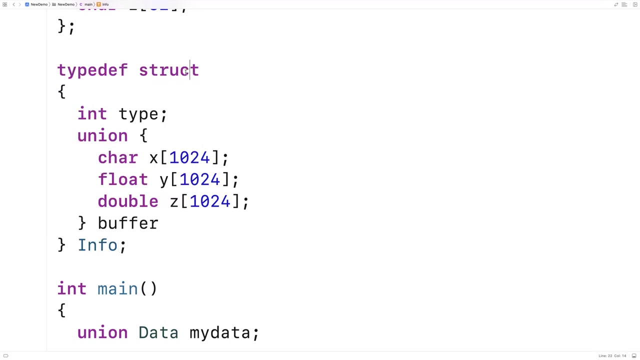 and we'll say int type union and we'll say car x 1024, float y 1024 and double z one thousand twenty four, and we'll call this union buffer and we'll call this typedef of a struct here info. so what i've got here is a union. 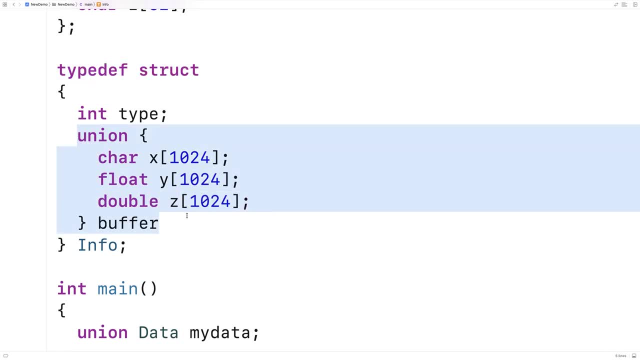 inside of a struct and it's a member of that struct, called buffer. here. with this type member, what i could do is set values that signify which union member is actively in use. so maybe type zero could signify that x is in use. type one could signify that y is in use. 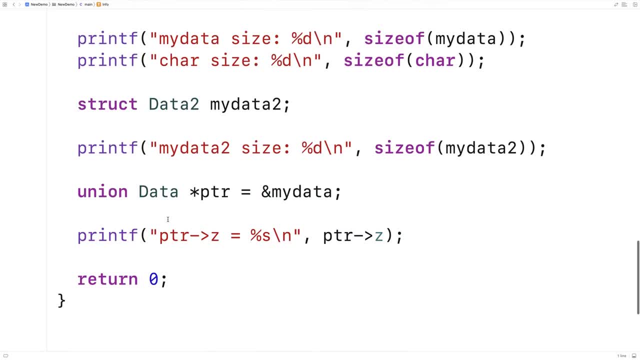 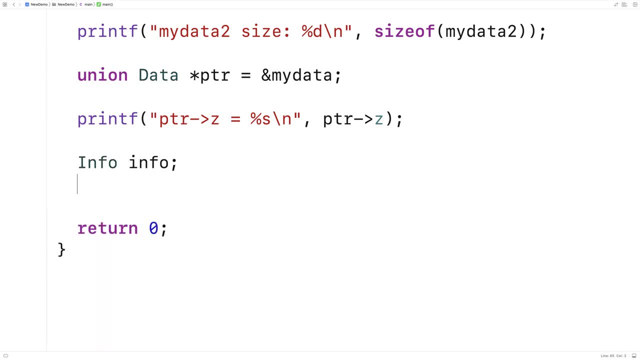 and type two could signify that z is in use. so we could then do things like this: we could say info, info, and then we could say infotype is equal to zero to signify that the x member of the union is what's in use, and then we'll say memset. 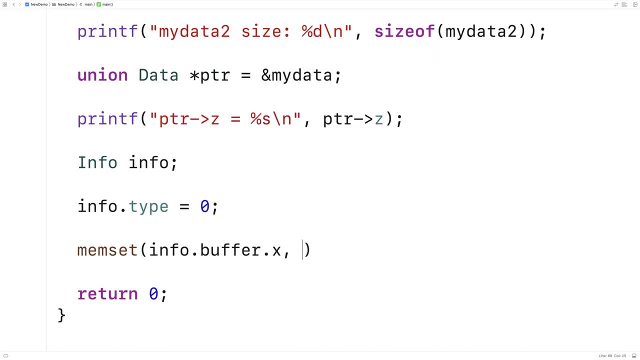 infobufferx set it to be all Ts for 1,024 characters And then we could do checks and we could check to see which member is in use before doing certain things. So we could say, like, if the infotype is zero, 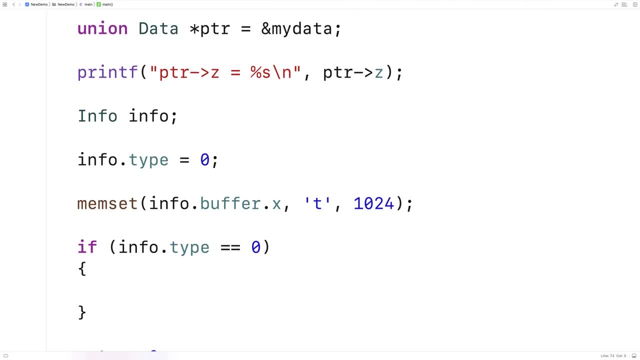 then we know that the X member is in use and we know, for example, that we could print out the characters in that buffer. So here we'll say: for int, i is equal to zero, i is less than 1,024, i++. 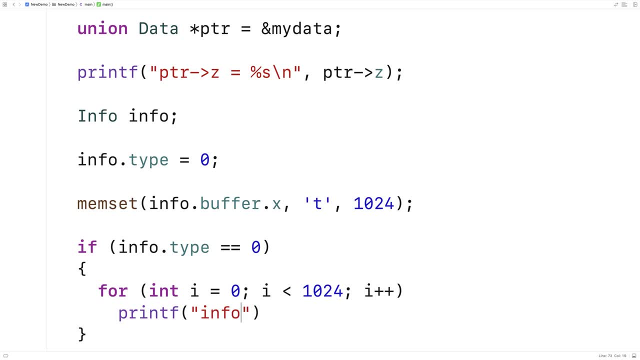 and we'll just print out all the characters in the buffer. So we'll say printf: infobufferx%d is equal to %c, slash n, and we'll output i and infobufferx at i. So if we save this and run it, 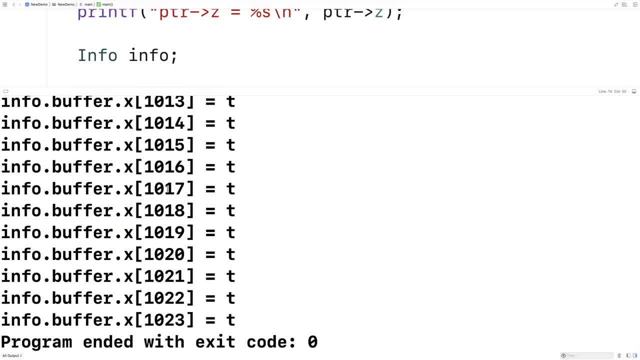 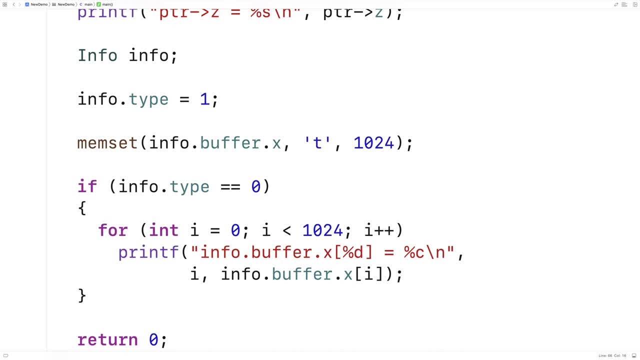 we should just print out all those Ts in that X member And then we can see that the Y member of the buffer union. but if, for example, the infotype was set to one, we'd be signifying that maybe the Y member is in use. 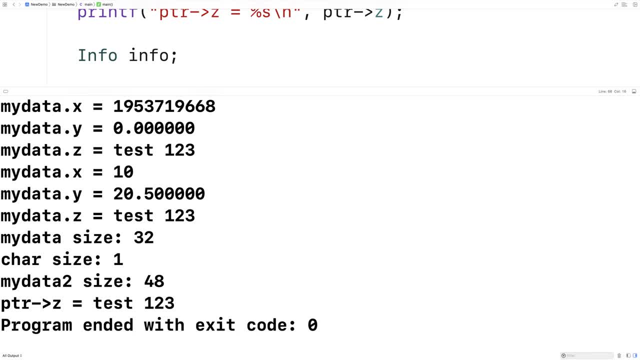 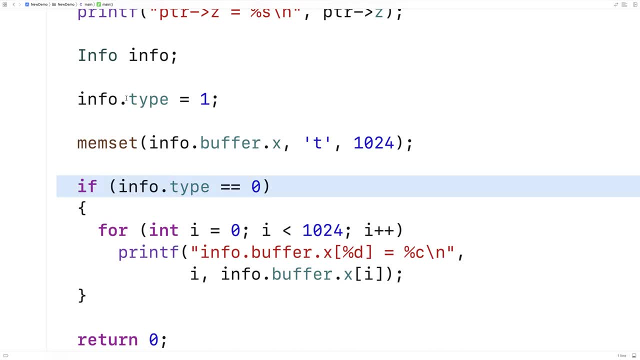 And then if we run this, we're never gonna print out the buffer values of the X member because the infotype is not zero. So we could use this type member of the struct to keep track of which of the union members is actually in use and then do or not do. 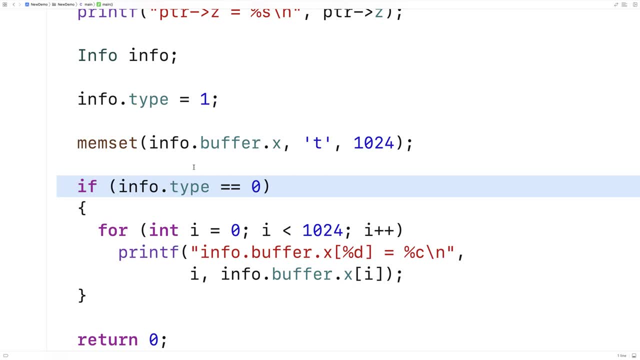 things based on what's in that union. So this is how unions work in C. We would typically use them in situations where memory is constrained, like, for example, inside embedded systems. I hope you enjoyed this tutorial. Thanks for watching. Check out PortfolioCoursescom. 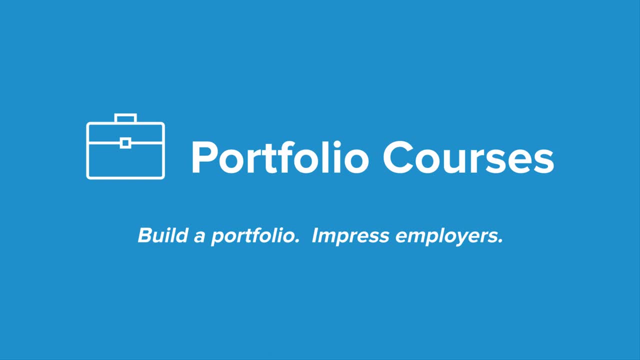 where we'll help you build a portfolio that will impress employers, including courses to help you develop C programming projects. 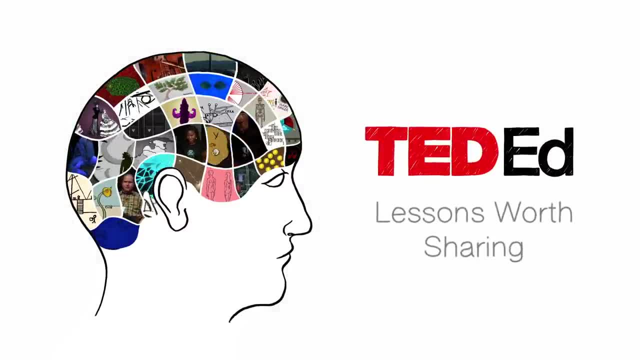 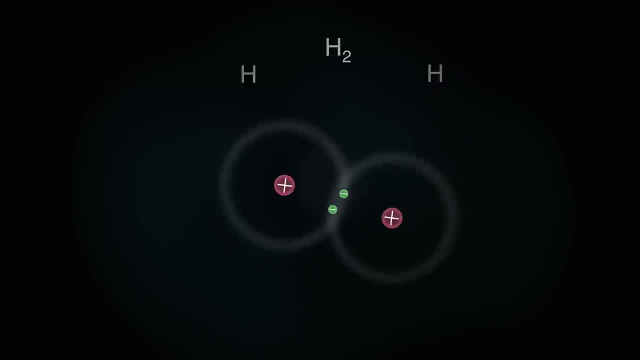 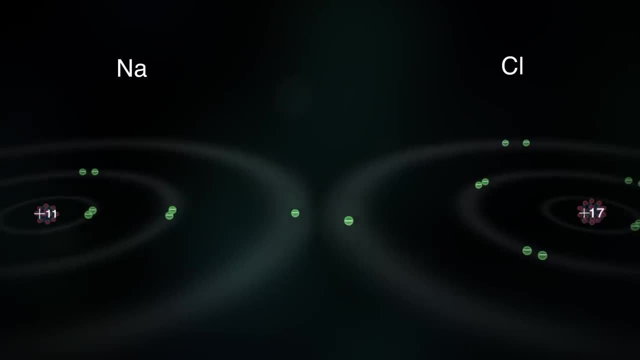 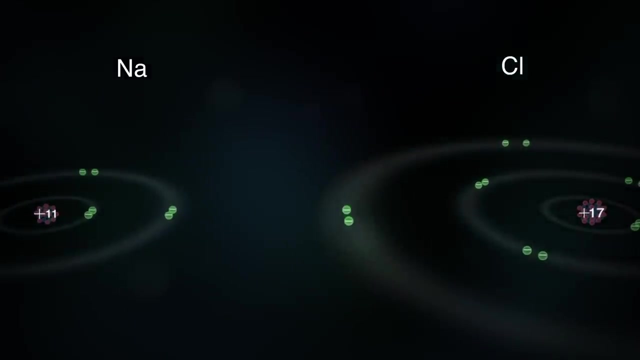 Most atoms don't ride solo. Instead they bond with other atoms. Now bonds can form between atoms of the same element or atoms of different elements. You've probably imagined bonding as a tug of war. If one atom is really strong, it can pull one or more electrons. 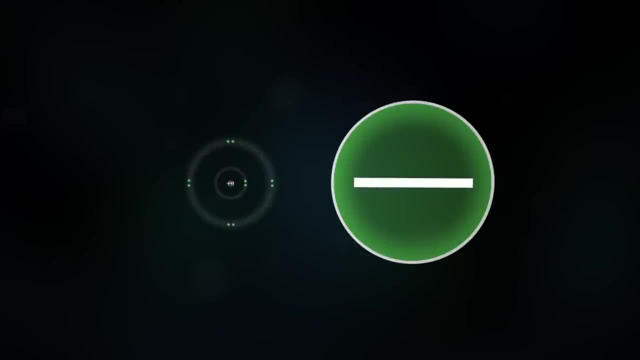 off another atom, Then you end up with one negatively charged ion and one positively charged ion, and the attraction between these opposite charges is called an ionic bond. This is the kind of sharing where you just give away your toy to someone else and then. 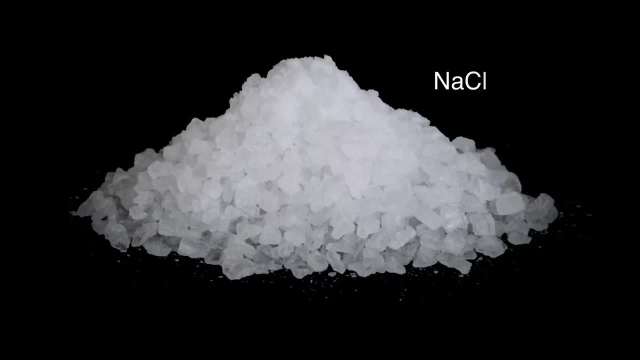 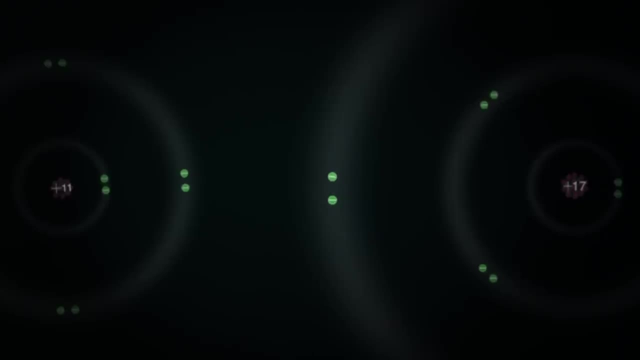 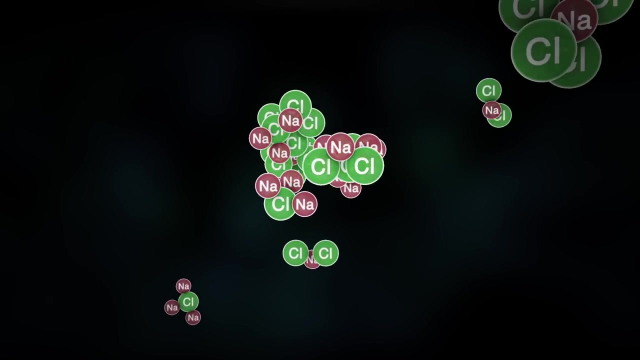 never get it back. Table salt, sodium chloride is held together by ionic bonds. Every atom of sodium gives up one electron to every atom of chlorine. Ions are formed and those ions arrange themselves in a 3D grid called a lattice, in which every sodium ion is bonded. 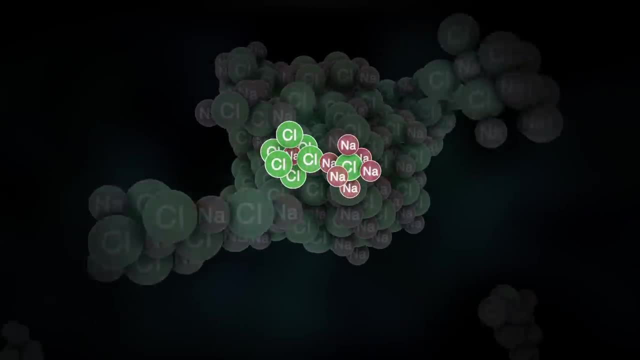 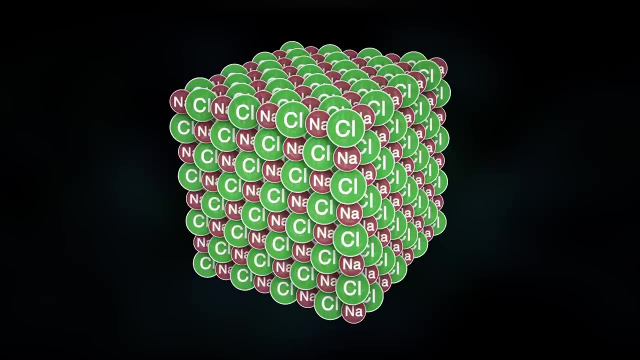 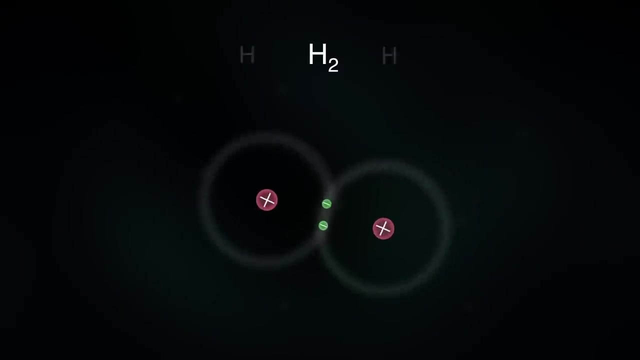 to six chloride ions, and every chloride ion is bonded to six sodium ions. The chlorine atoms never give the sodium atoms their electrons back. Now these transactions aren't always so cut and dried. If one atom doesn't completely overwhelm the other, they can actually share. 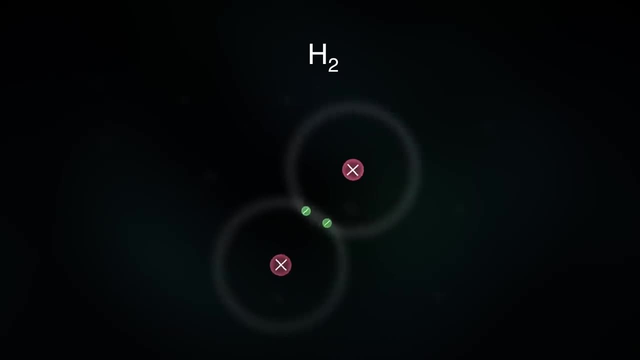 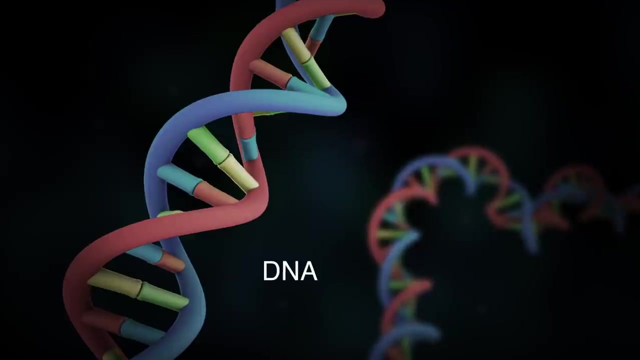 each other's electrons. This is like a potluck, where you and a friend each bring a dish and then both of you share both dishes. Each atom is attracted to the shared electrons in between them, and this attraction is called a covalent bond. The proteins and DNA in our bodies, for example, are held together largely.